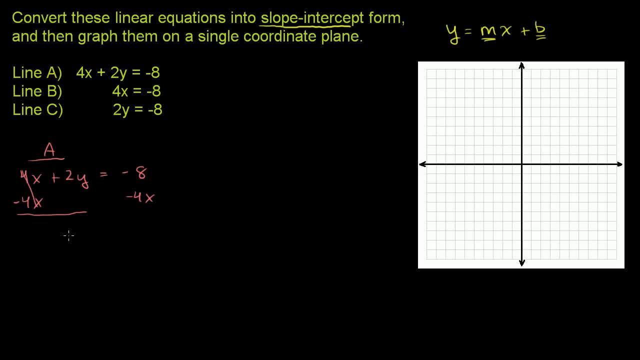 The left-hand side of the equation, these two 4x's cancel out And I'm just left with mx. I'm left with 2y is equal to, and on the right-hand side, I have negative 4x minus 8, or negative 8 minus 4x. however, 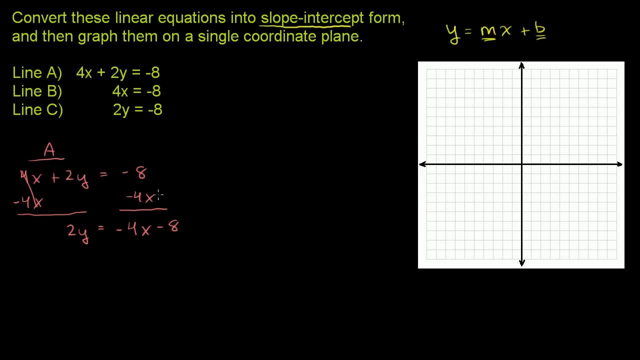 you want to view it Now. we're almost at slope intercept form. We just have to get rid of this 2. And the best way to do that that I can think of is divide both sides of this equation by 2.. 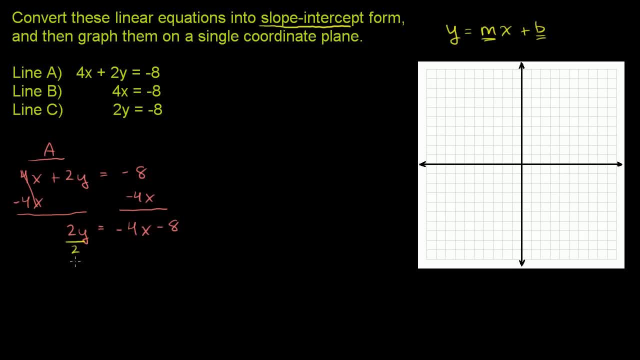 So let's divide both sides by 2.. So we divide the left-hand side by 2, and then divide the right-hand side by 2.. You have to divide every term by 2.. And then we are left with: y is equal to negative 4 divided by. 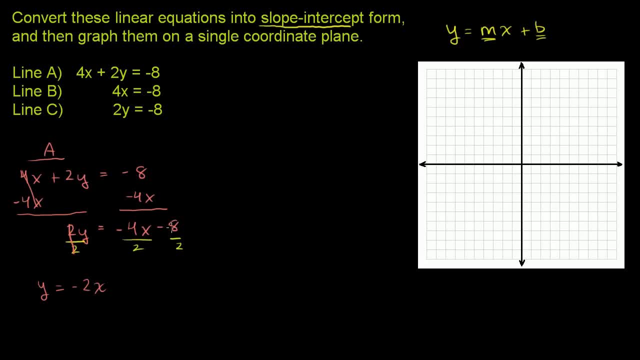 2 is negative, 2x Negative. 8 divided by 2 is negative 4.. Negative 2x minus 4.. So this is line a And let me graph it right now. So line a, its y-intercept, is negative 4.. 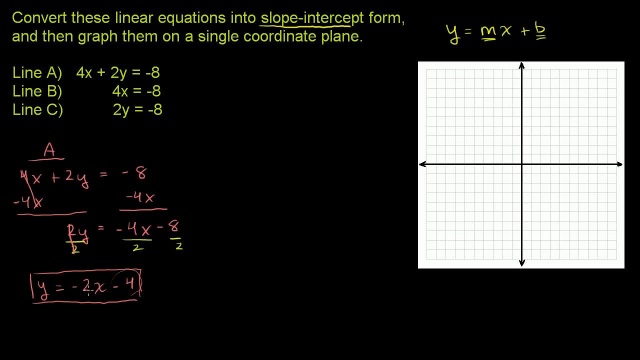 So the point 0, negative 4 is on this graph. if you actually look at the y-intercept, you can see that y is equal to 0, y is going to be equal to negative 4.. You can just substitute that in the graph. 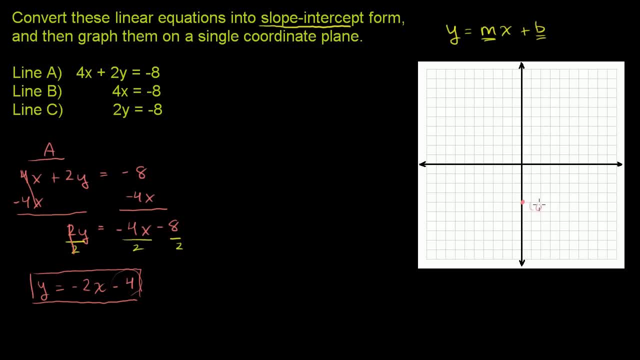 So 0,, 1,, 2,, 3,, 4, that's the point. 0, negative 4.. That's the y-intercept for line a, And then the slope is negative 2x. So that means that if I change x by positive 1, that y goes. 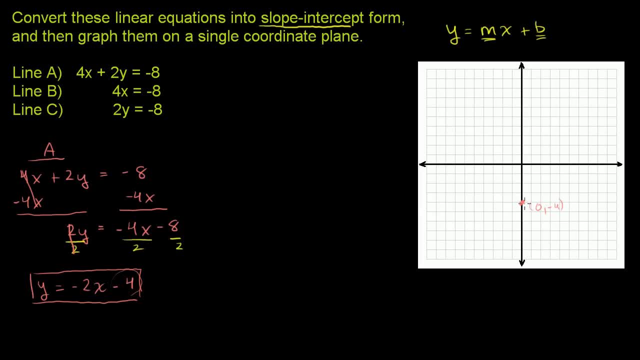 down by negative 2.. So let's do that. So if I go over 1. In the positive direction, I have to go down 2.. That's what a negative slope is going to do. Negative 2 slope: If I go over 2, I'm going to have to go down 4.. 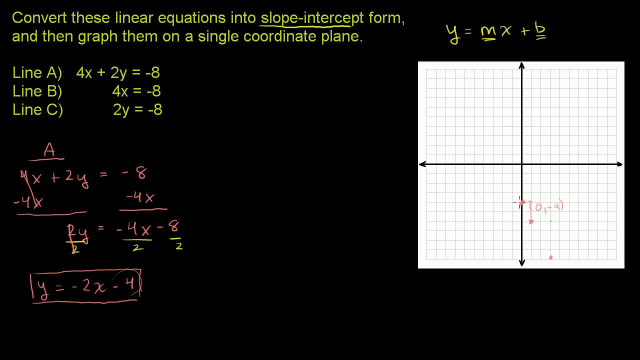 If I go back negative 1, so if I go in the x-direction negative 1, that means in the y-direction I go positive 2. Because 2 divided by negative 1 is still negative 2.. So I go over here. 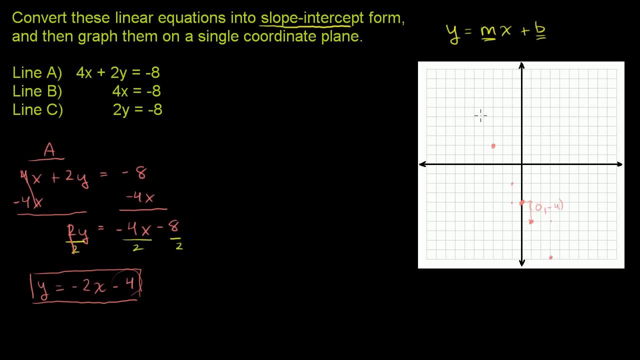 If I go back 2, I'm going to go up 4.. Let me just do that a couple of times: Back 2 and then up 4.. So this line is going to look like this. This line is going to look like this: 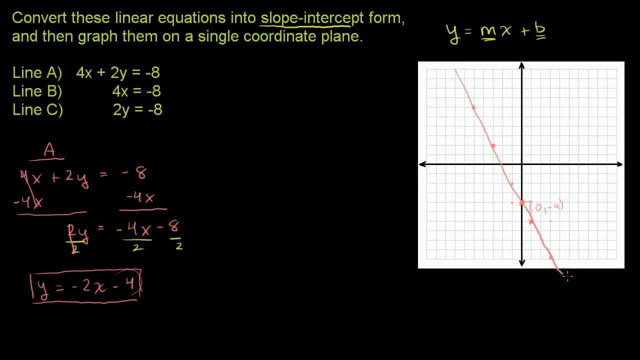 I'll do my best to draw it. That's a decent job. That is line a, right there. All right, let's do line b. They say 4x is equal to negative 8.. And you might be saying, hey, how do I get that into slope? 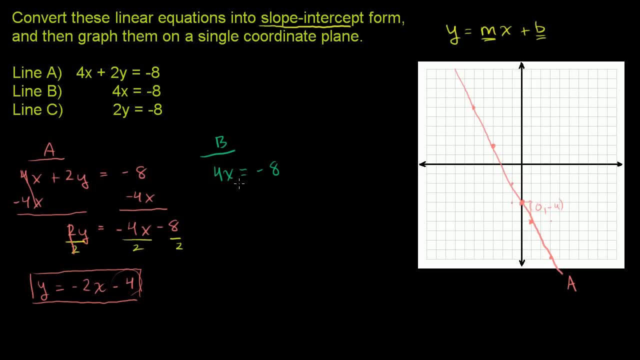 intercept form. I don't see a y And the answer is: you won't be able to Because this can't be put into slope intercept form. but we can simplify, So let's divide both sides of this equation by 4.. 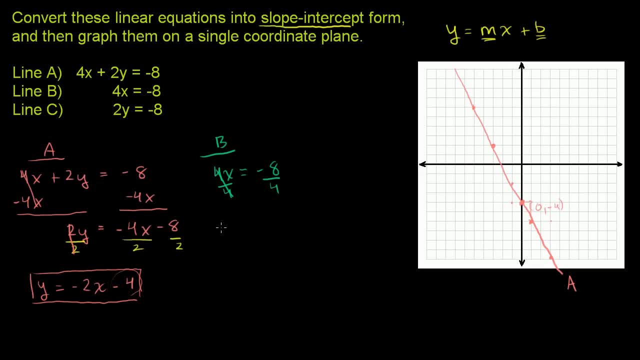 So you divide both sides of this equation by 4. And you get x is equal to negative 2.. So this just means I don't care what your y is, x is just always going to be equal to negative 2.. So x is equal to negative. 2 is right there. 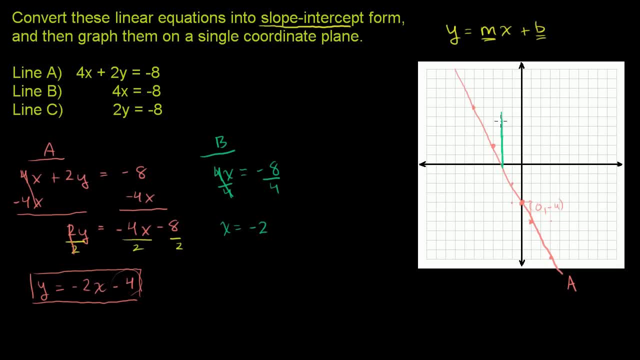 Negative 1, negative 2.. And x is just always going to be equal to negative 2.. x is always going to be equal to negative 2 in both directions, And this is a bit of a review. This is the x-axis. 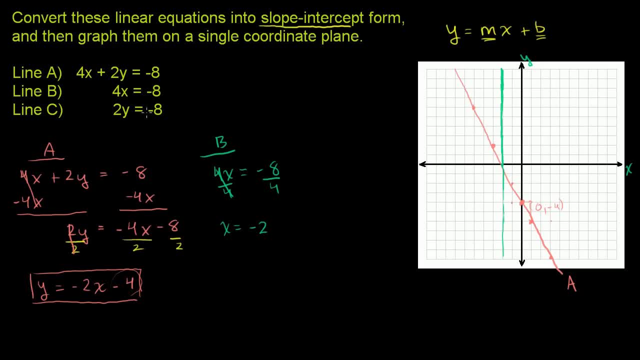 That's the y-axis. I forgot to label them. Now let's do this. last character, 2y, is equal to negative 8.. So line c We have: 2y is equal to negative 8.. We can divide both sides of this equation by 2.. 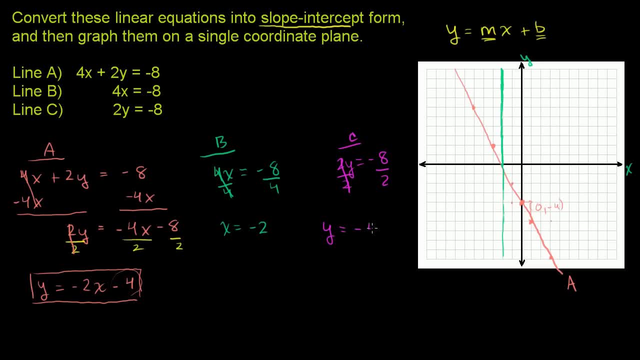 And we get: y is equal to negative 4.. So you might say: hey, Sal, that doesn't look like this form, slope intercept form, But it is. It's just that the slope is 0.. We could rewrite this as: y is equal to 0x minus 4, where the 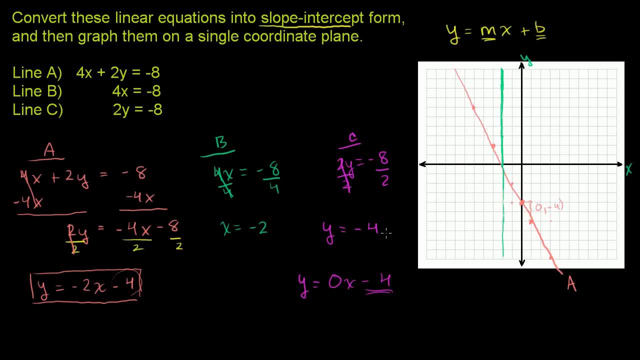 y-intercept is negative 4 and the slope is 0.. y-intercept is negative 4, right there, And the slope is 0.. So if you move an arbitrary amount in the x-direction, the y is not going to change. 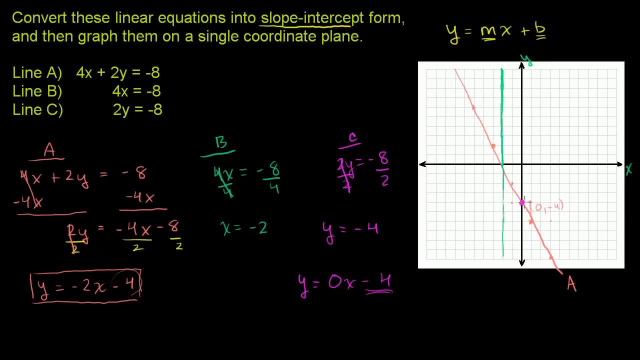 It's just going to stay at negative 4.. Let me do that a little bit neater: y is just going to stay at negative 4.. Or you could just interpret it as: y is equal to negative 4, no matter what x is. So then we are done.